especially model fractured networks, rely only on the histograms or basically the distribution of the fracture length and the distribution of the fracture orientation or strike angle. So the idea is that if we know the distribution of the fractures in terms of the length and the orientation, that should be good enough to make or generate a representative model of the fracture networks in the subsurface. But it turns out that's not accurate Because, for example, in this zone of Q3ration here there's two pronounced fractures between four of the mes rivalizers and the nephrop volont 끖s. these are now three scattered structural factors, and these are also Nh 경 nge싱, queimig bi tomci, Erram as the selecting product and espy respiratory level. And this would stupidати us that if we collected new rapeez, we 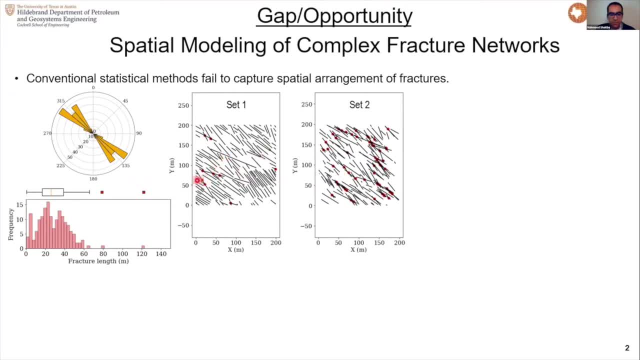 For example, in this example, these two fracture sets, set one and set two, have the exact same distribution for fracture length, shown on the left hand side, and the same rose diagram and the distribution for the orientation, But, as you can see, they have completely different spatial characteristics. In set two, fractures are connected over the entire study domain. the connections between fractures, or the intersection points, are shown with red dots. 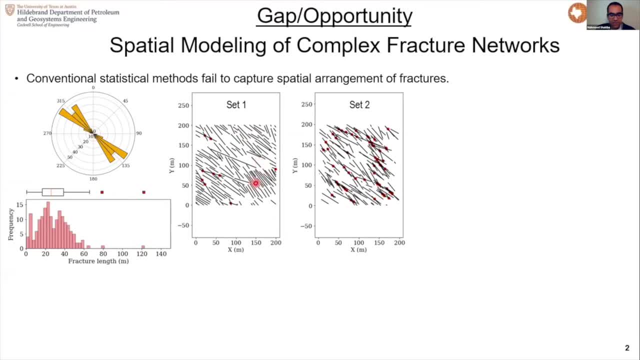 But the set number one on the left hand side. it has only a few intersection points or the connectivity is much lower than set two. So although they have the same distribution in terms of histograms, they exit with different spatial characteristics. The same problem exists for 1D application as well. 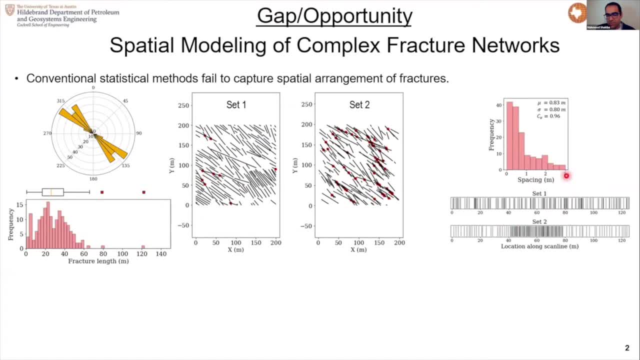 So these two fracture sets, set one and set two, they have the same or exact same distribution for spacing between fractures. But, as you can see, set one is more or less randomly distributed, but in set two we have a major cluster in the middle. 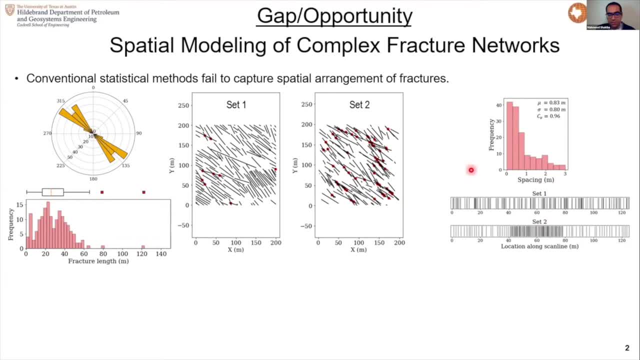 So some of the conventional statistical measures that are often used in the industry, such as histograms, actually fail to capture the spatial distribution of the fractures in the subsurface. Another complexity with modeling fracture networks is that they exhibit multi-scale size distributions. So if you plot, for example, the spacing between fractures or fracture apertures, 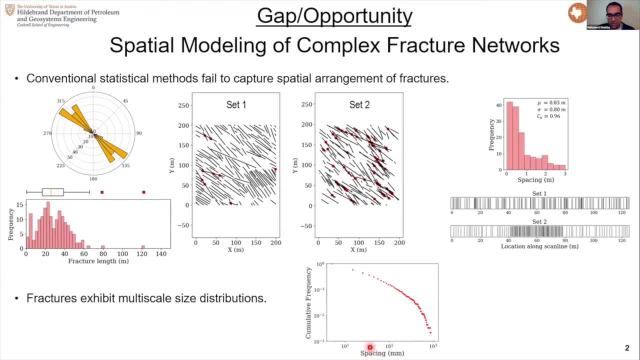 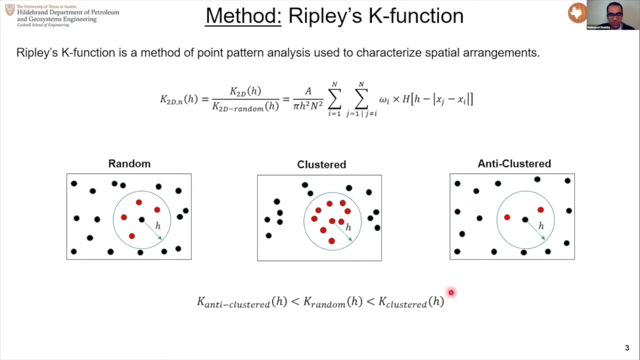 or fracture length. often you see that they span across multiple length scales. So the statistical methods that we use, they should not only consider the spatial arrangement of the fractures but they should also be a multi-scale method. So to address those issues we have used a method called the Ripley's k function. 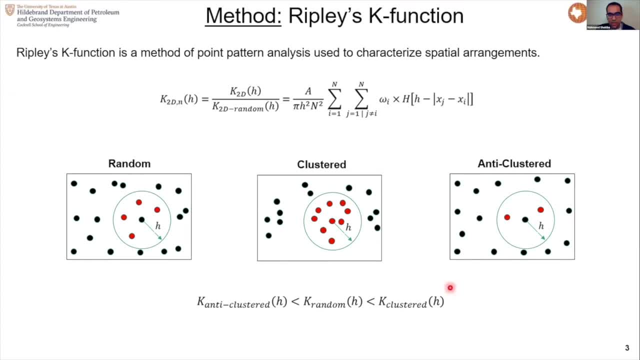 Ripley's k function is a method of point pattern analysis that primarily applies to the distribution of discrete points Or discrete events in the space, And we can use Ripley's k function to characterize a spatial organization of fractures in the subsurface. So here is the formulation shown here: 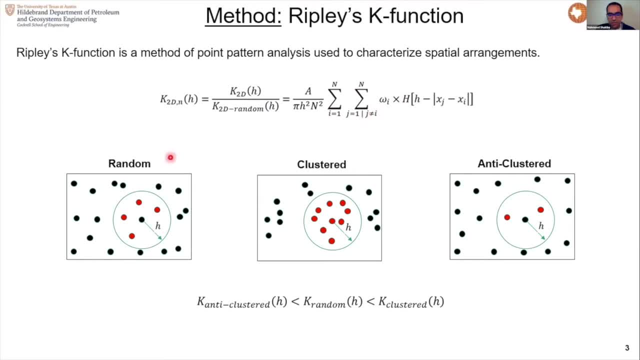 So basically, what it estimates is the expected number of points that fall within a search area that put on a random point inside a study domain. So if we know the area of the search area and if we know the intensity of the points, we know how many points are in the study domain. 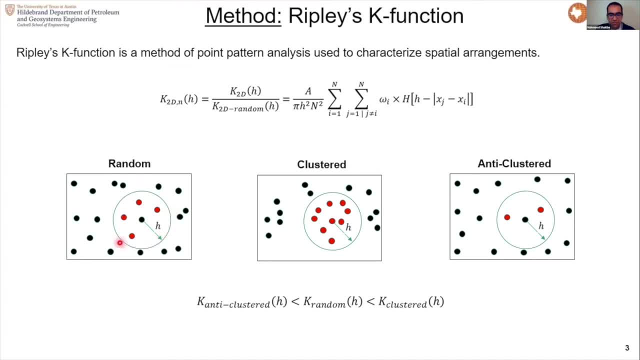 So if we know the area of the search area and if we know the intensity of the points, we know how many points we should expect to see inside this circle. So if the number that we calculate using this equation for a specific pattern, if the number of neighbors is larger than what we expect to see from a random, 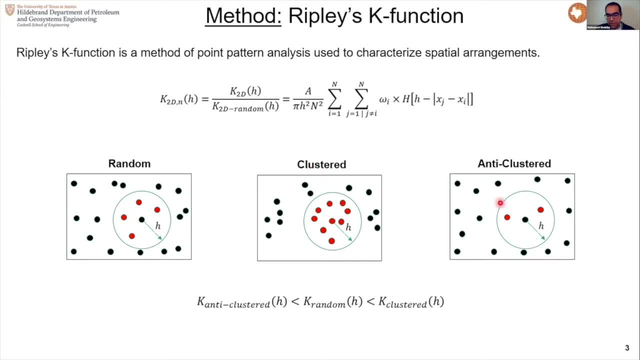 then we call that a spatial pattern cluster. If the number of neighbors is less than what we expect to see from a random distribution, then we call that pattern anti-cluster. So there's always a comparison made between what we calculate based on k function and what we expect to see from a random distribution. 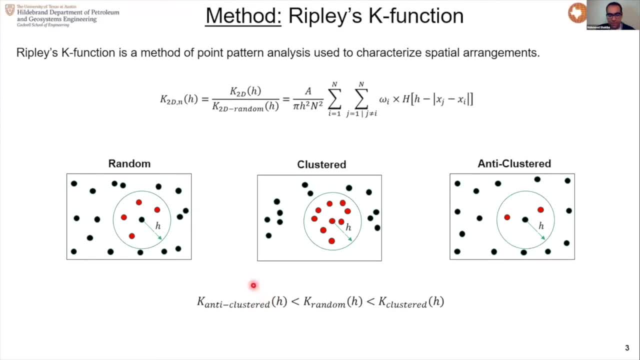 The nice thing about a Ripley's k function is that we can do the analysis. we can perform a multi-scale analysis. So if we change the size of the circle, we can do the same calculations at another scale and we can see if, for example, clustering or anti-clustering changes from one scale to another. 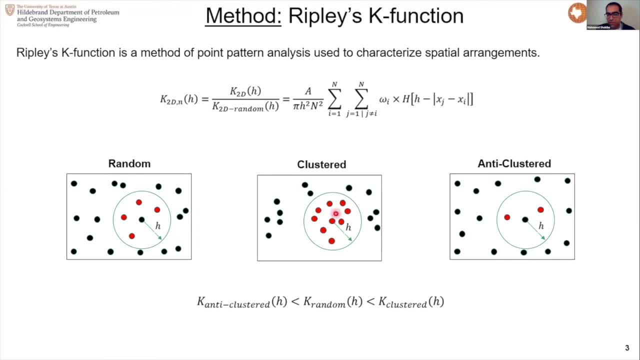 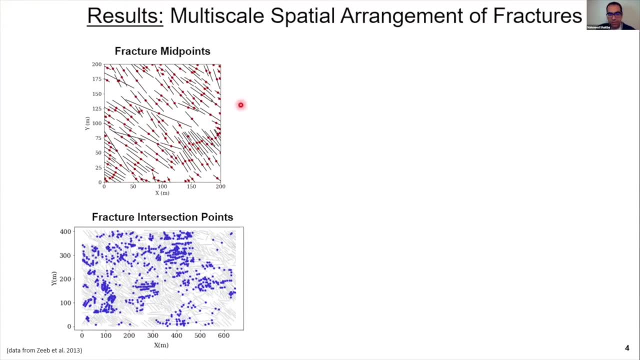 So, as you can see, this method applies to data points, So before we can use it for fractures, we have to convert the fracture network to point patterns. There are several options. One of them is to replace fractures with the barycenters or midpoints. 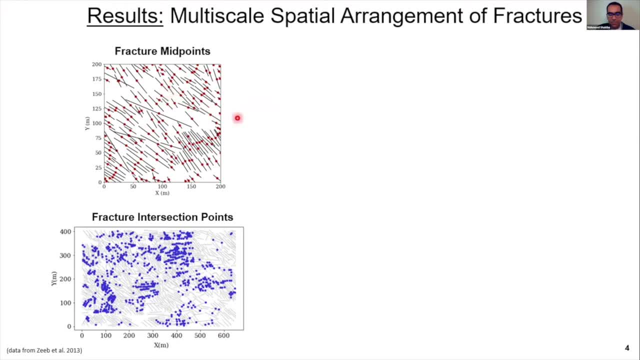 So when we replace fractures with the barycenters, so the distance between the midpoints actually provides some information on how close the fractures are inside the network. Another approach is to use the fracture intersection points, So whenever two fractures cross each other or converge, 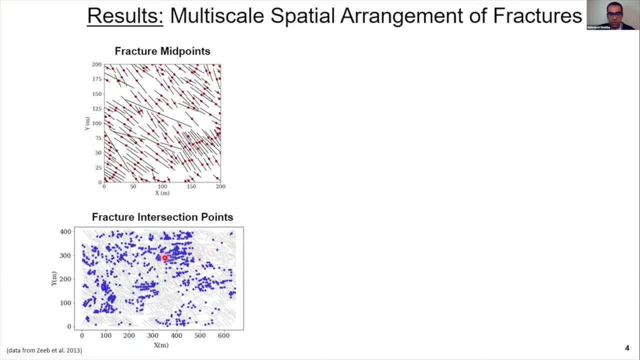 and intersect. we can put a point and then replace the whole fracture network with distribution of intersection points inside the study domain. The advantage of looking at the spatial distribution of the intersection points is that it provides some information on the degree of connectivity over the entire study domain. 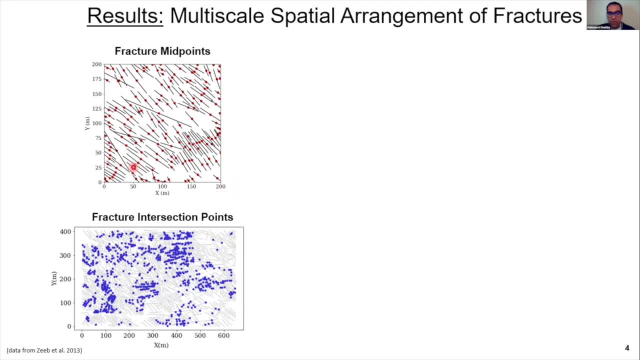 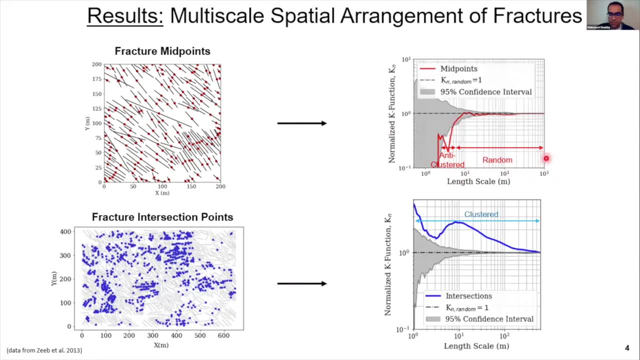 Now that we have converted the fracture network to points, we can go ahead and apply the k function formulation to get figures like this. Let me explain how to interpret these figures. So on the x-axis we have the length of scale that goes from 1 to 1000 meter. 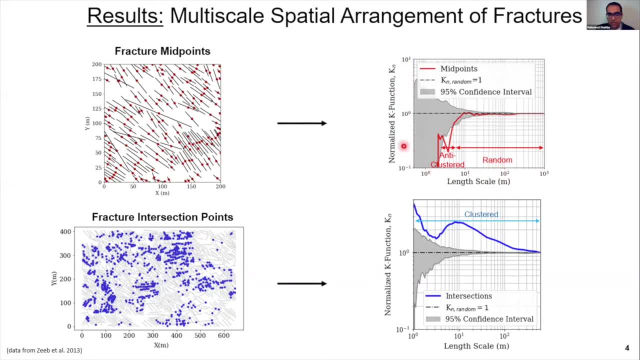 And on the x-axis. on the y-axis we have the normalized k function. The shaded region is the confidence interval for a random arrangement. So if the line falls inside the shaded region then the distribution is not distinguishable from random. But if it falls outside of the shaded region, 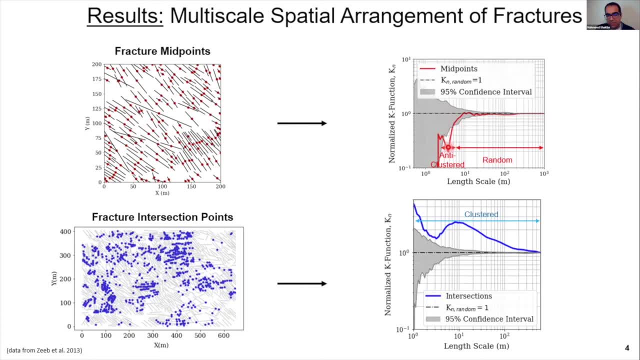 for example in this section, then the spatial organization is statistically significant. So for example, for the fracture midpoint at length of scale less than 5 meter in this part we can see that the red line falls outside of the shaded region. 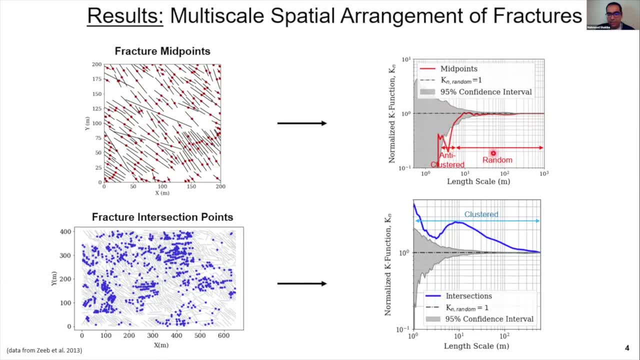 So the distribution is anti-clustered. At other length of scales it's inside the shaded region, so it's random. When we look at the fracture intersection points in the second example, we can see that the line is always above the confidence interval. 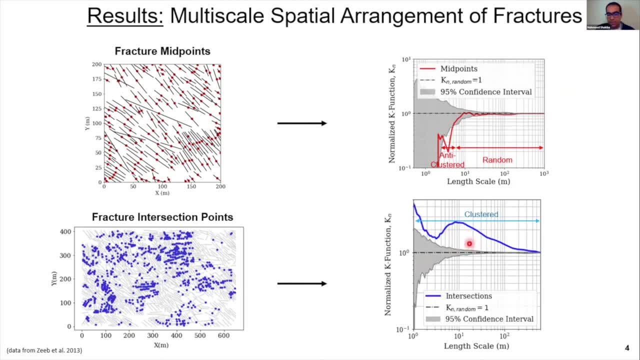 So we can say that this specific pattern is clustered across all the length scales that we are interested in. So using the replace k function provides an opportunity to perform a multi-scale characterization of fractures to see if they are random, clustered or anti-clustered. 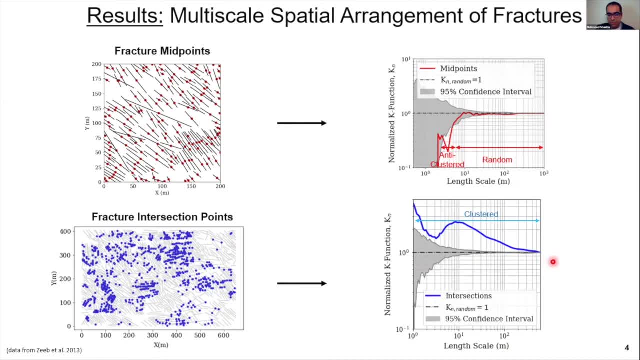 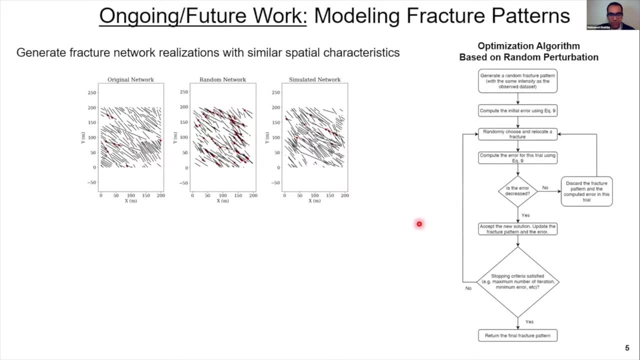 We can also use this information to model fractures or to generate fracture network realizations. So this is an ongoing part of the project, but I have some preliminary results to show. So this is the fracture networks that I showed in the first slide. So they have the exact same fracture segments. 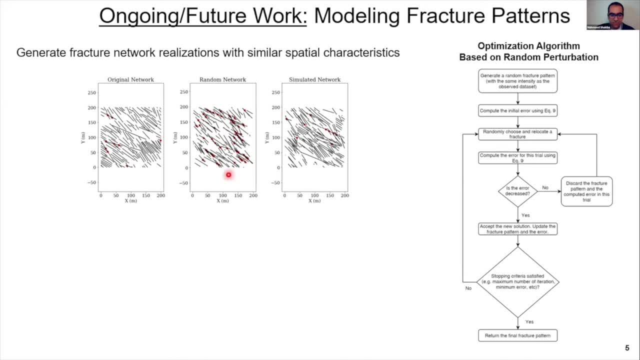 but they exhibit different spatial characteristics. The fracture network, which is distributed randomly. you can see a lot of red dots and red dots are the intersection points. So the degree of connectivity is much higher in the random network than the original network on the left-hand side. 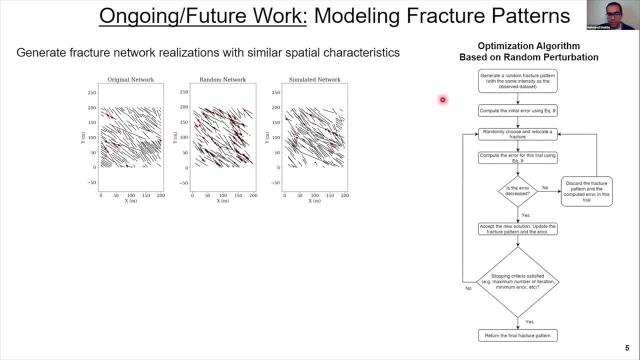 So we developed an optimization algorithm based on random perturbation, which is shown on the right-hand side. The way that this optimization algorithm works is that we take the random network, the initial random network, and at each iteration step we perturb the location of the fractures. 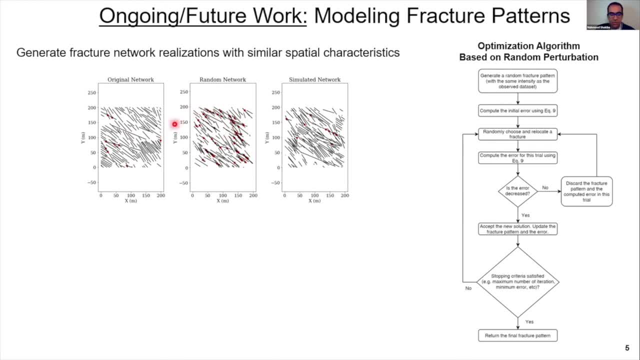 We calculate the k function at various length scales and then we compare it with the original network. If the mismatch is reduced, then we accept the new arrangement. If not, then we ignore it and we move on to the next iteration. We perform another perturbation. 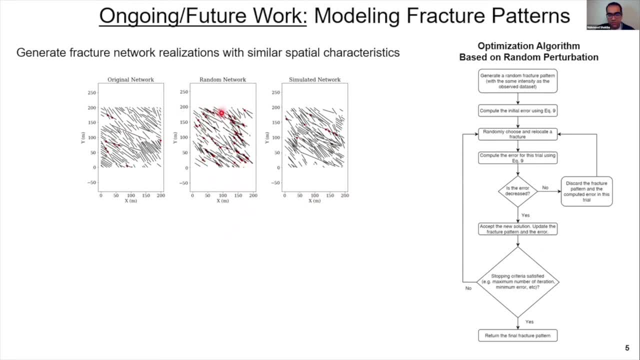 So at the end we can convert the random network to a simulated network which has the same spatial distribution of the fracture intersection points as that of the original network. Here is another example. So in the original network most of the intersection points 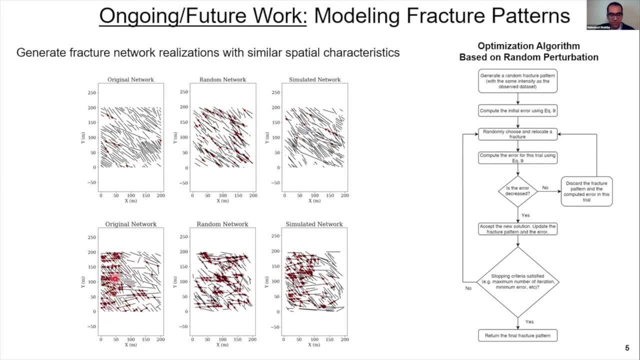 shown with the red dots are clustered on the left-hand side, But if you randomly distribute fractures you can see that the intersection points are distributed over the entire study domain. But again, if we use the optimization algorithm we can generate a simulated network. 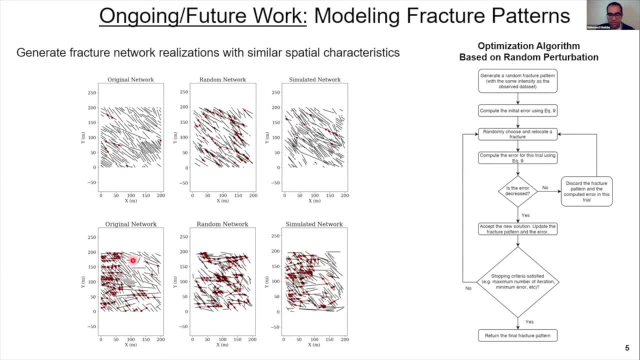 which has spatially similar characteristics as that of the original network. So now that we know that the points, or intersection points or the midpoints are spatially distributed similar to the original network, we have to make sure that they produce the same flow behavior. 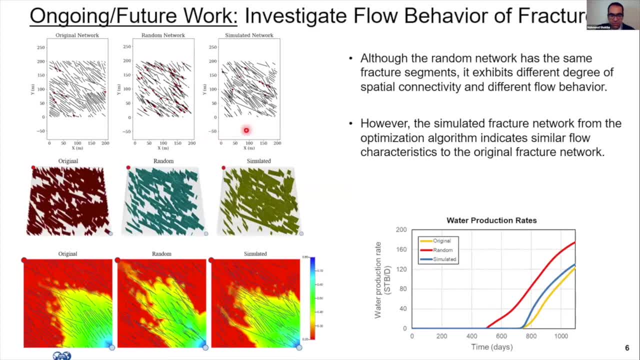 So what we are proposing is to convert the fracture networks or construct discrete fracture models for the original network, for the random network and for the simulated network. Then we run synthetic flow simulation models. So, for example, in this case I have an injection. well, 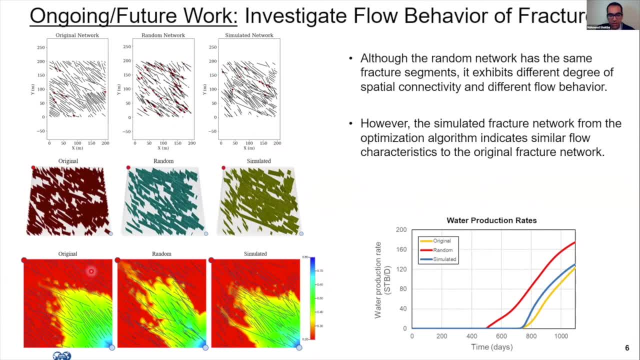 located on the lower right corner and a production well located on the upper left corner of the simulation models And after a specific number of simulations you can see that in the random network the water has already reached the production well because of the higher degree of connectivity. 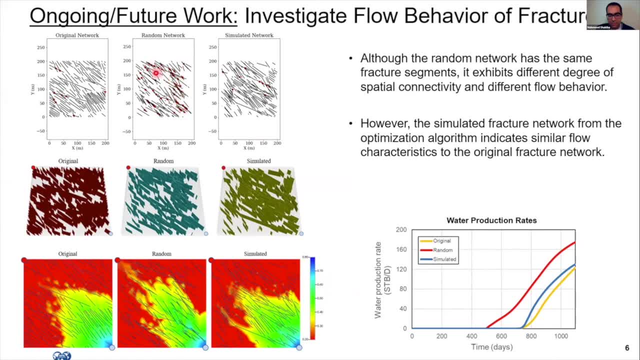 between fractures, as are evident in this picture. But in the original and in the simulated fracture network the waterfront is still far away from the producer, And this is also evident from the water production rates, in which the water breakthrough occurs earlier than the other two network model. 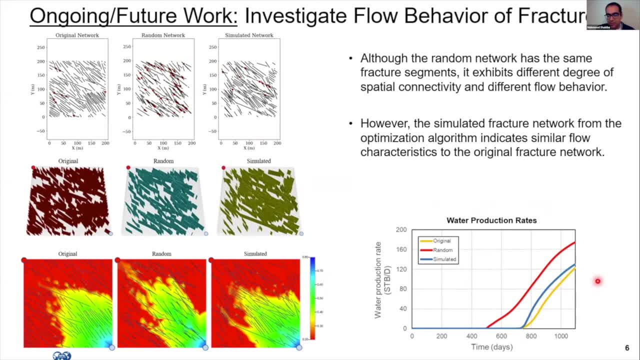 So, to summarize, using methods like Ripley's k function, we can characterize the spatial distribution of the fractures to see if they are random, clustered or anti-clustered, And you can also use that information to generate representative or spatially similar fracture network realizations. 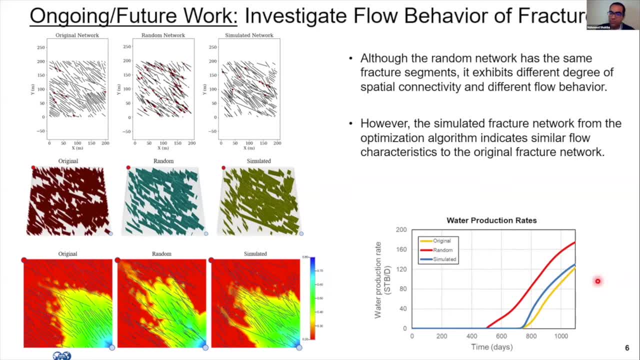 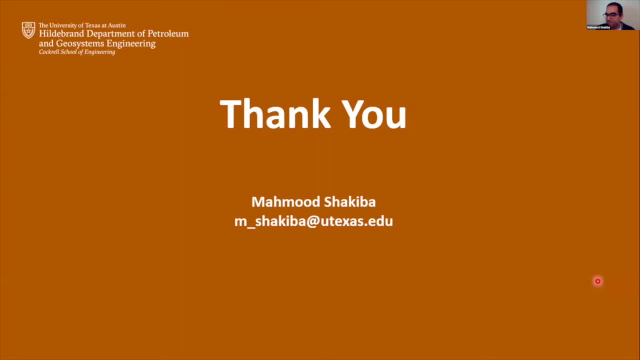 for further uncertainty analysis or other modeling purposes. With that I finish the presentation and I would be happy to answer your questions. Thank you for your time. Thank you, Mahmoud. thank you very much. I appreciate your talk and appreciate you, Mahmoud. I want to give you full credit. 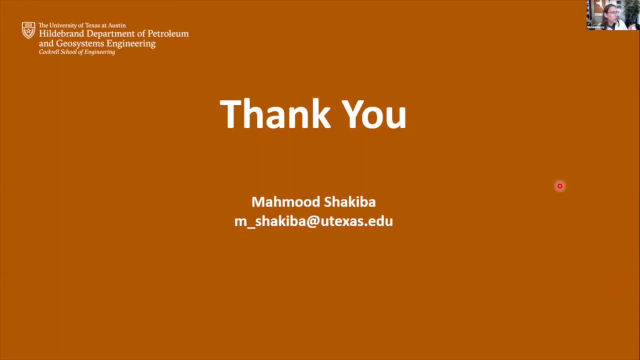 You weren't originally on the schedule and you said I would really like to show this work this week and you just jumped right to it. This is a great presentation. I appreciate you jumping in and showing the initiative. Thanks for the opportunity. Any questions from any of our participants? 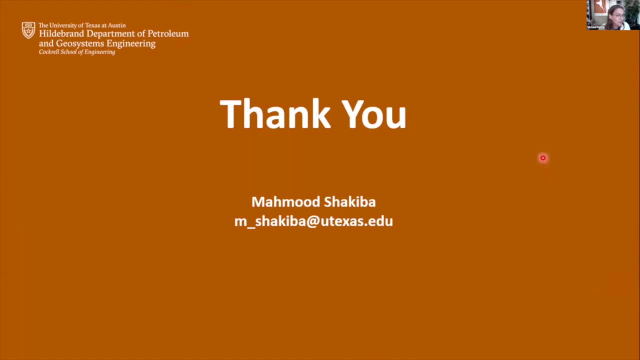 You know I'm going to ask a question if nobody else does. What about? there's spatial point processes and then there's marked spatial point processes. A marked spatial point process includes not only spatial location but also information like orientation and aperture. Have you given any thought? 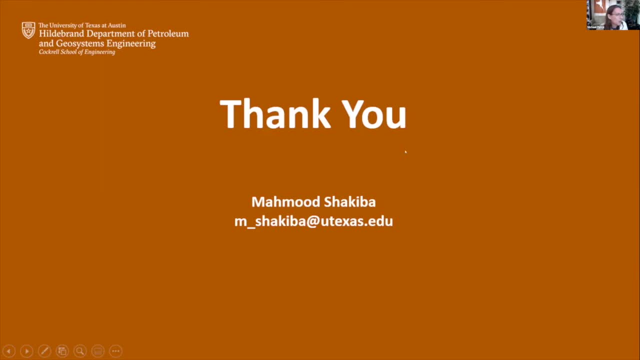 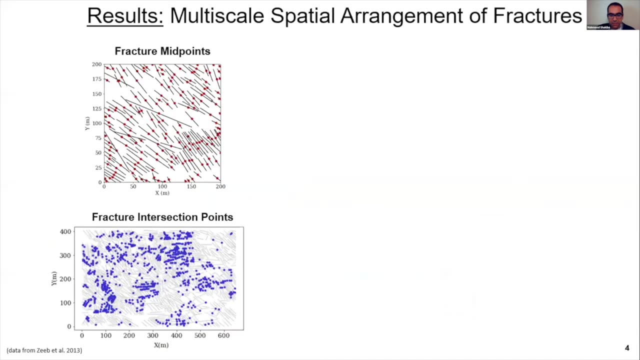 to incorporating in the model orientation aperture other types of features? Yes, So if I go back, let me see if I can. So if you look at, for example, these data points, they don't have any mark or label. 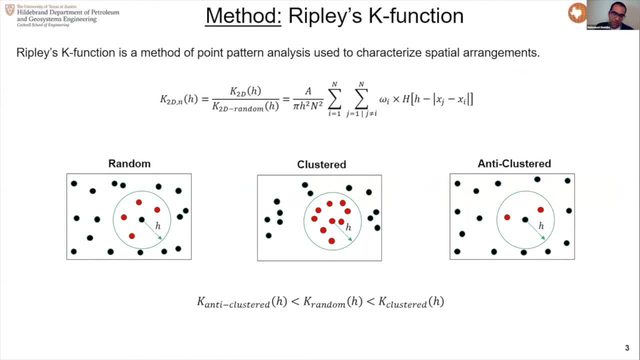 So one of the approaches that we have used- and actually we have prepared the manuscript to submit to a journal- is that we can classify the data points or fractures based on the attribute that we're interested in, For example, if there's a threshold for aperture size. 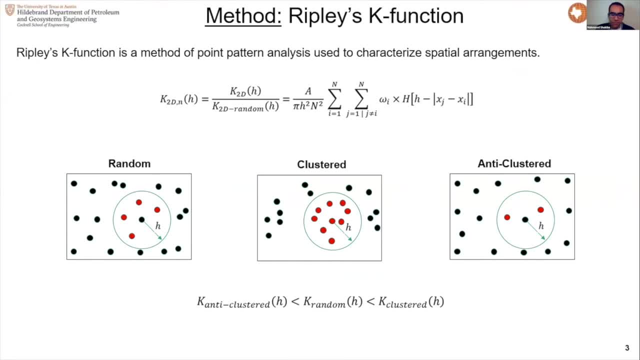 we can create two different classes or if one of the some of the fractures are like propped, some of them are open, we can generate different classes and we can perform the same spatial analysis on different classes to see if there is any attraction or repulsion, so to speak. 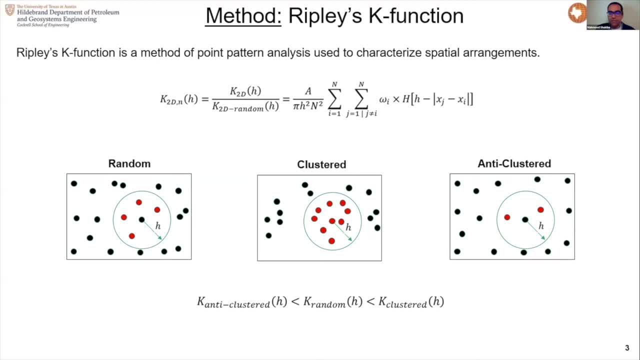 between the fractures from different classes. So that would, instead of you know, giving us information about clustering and anti-clustering, we can see if there is any attraction or synchrony or any repulsion or asynchrony between the different fractures from different classes or different sets. 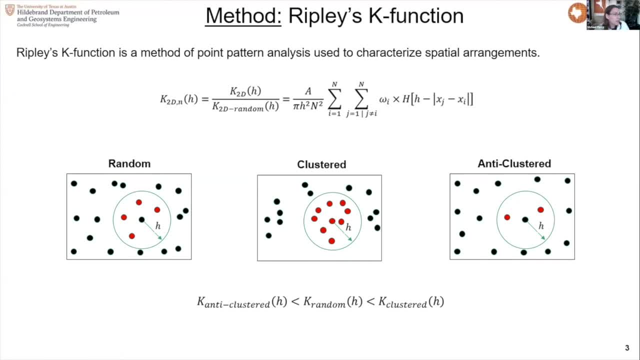 And we might find out that there is no relationship. Yeah, yeah, exactly. I have to say, one of the great things about this type of extension- you use the spatial data analytics- is the fact that you'll find out often that there is not a significant relationship. 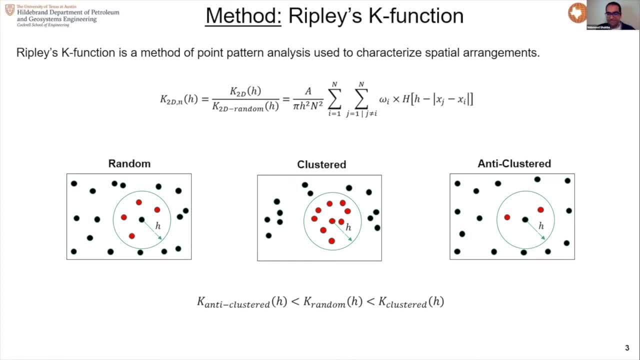 Correct. yeah, I think our eyes, our brains, that have evolved over so many- you know, hundreds of thousands of years, are very good at finding patterns at random Exactly. yeah, Yeah, You can avoid making that mistake, All right, any questions? comments? Mahmoud, thank you very much. Appreciate it. Thank you so much. 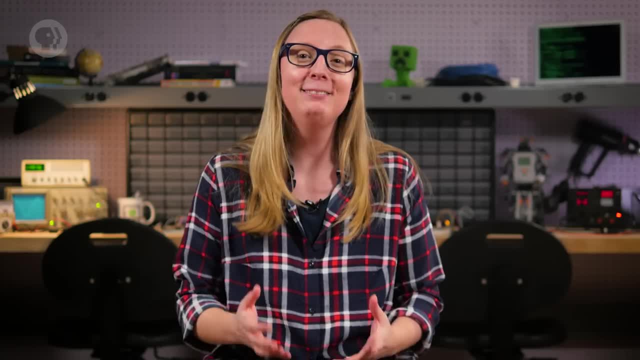 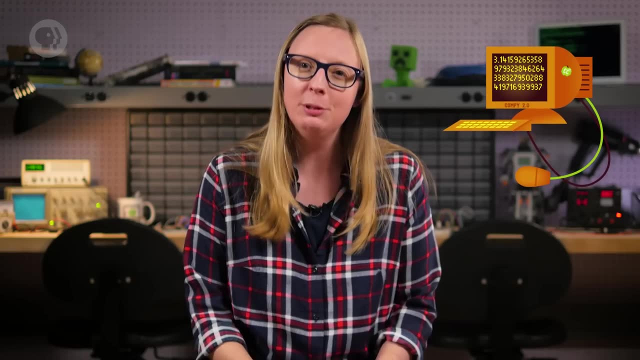 Hi, I'm Carrie-Anne and this is Crash Course, Computer Science, and today we're going to talk about how computers store and represent numerical data, which means we've got to talk about math, But don't worry, every single one of you already knows exactly what. 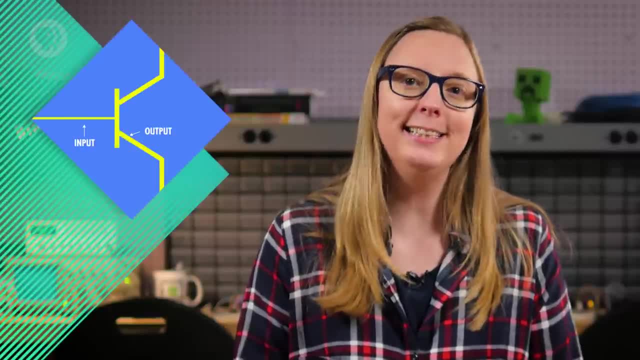 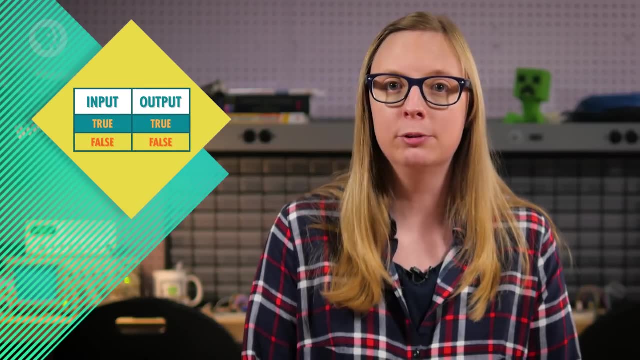 you need to know to follow along. So last episode we talked about how transistors can be used to build logic gates which can evaluate Boolean statements. And in Boolean algebra there are only two binary values: true and false. But if we only have two values, how in the world do we represent information? 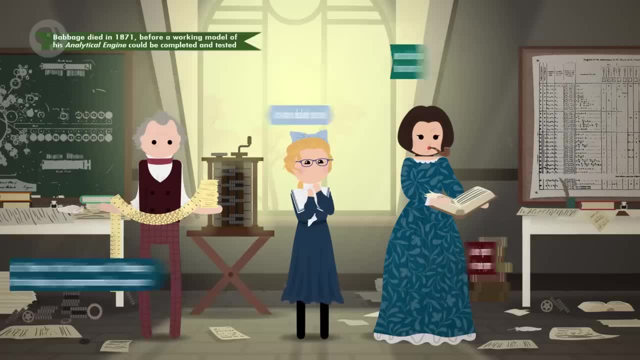 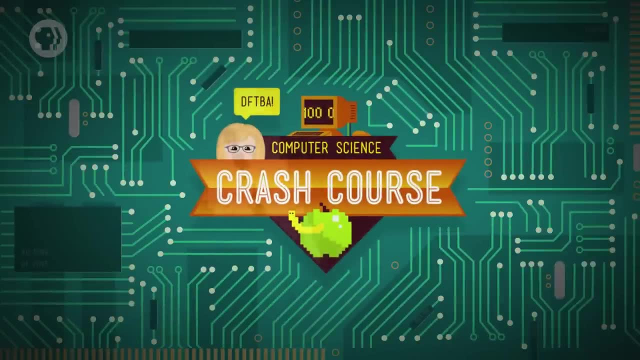 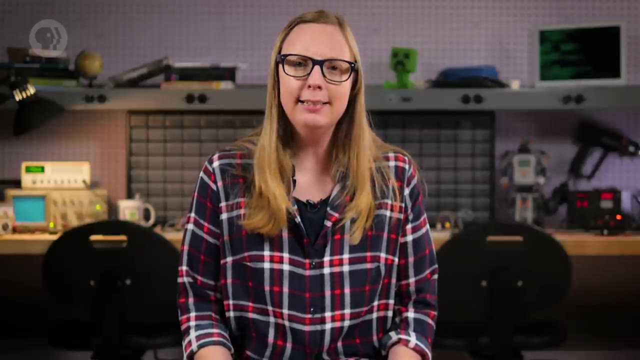 beyond just these two values. That's where the math comes in. So, as we mentioned last episode, a single binary value can be used to represent a number. Instead of true and false, we can call these two states 1 and 0,, which is actually incredibly. 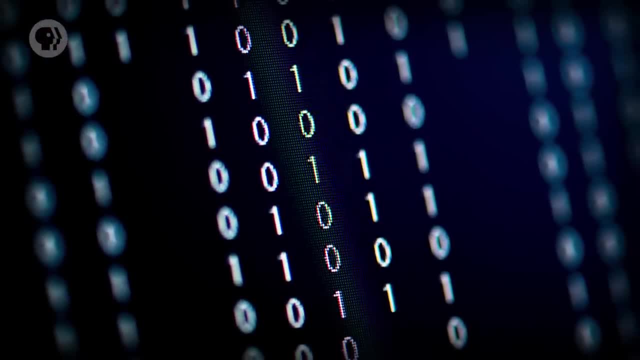 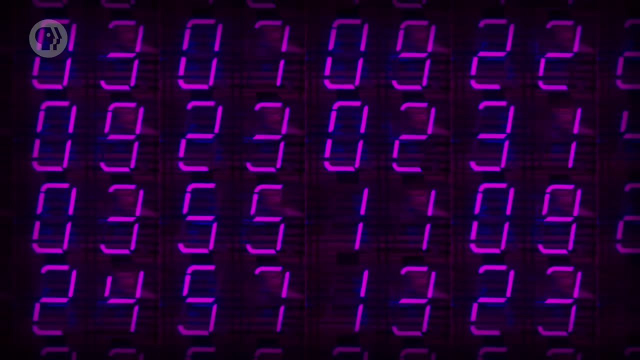 useful, And if we want to represent larger things, we just need to add more binary digits. This works exactly the same way as the decimal numbers that we're all familiar with. We've got a few numbers here. For decimal numbers, there are only 10 possible values. a single digit can be 0 through 9..